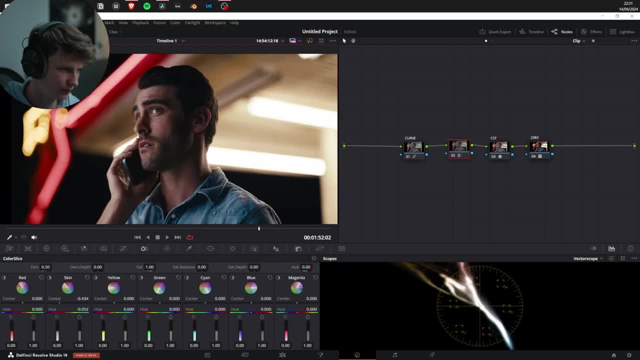 They're perfectly on the line, but in my opinion maybe a little bit more red and slightly more saturated. We also remove slightly some of the density on the skin tones because they were a bit too dark. We add a slight bit of the density to the red because the red looks really nice when dense. 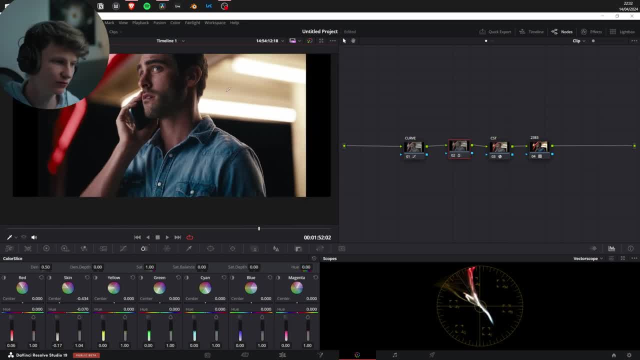 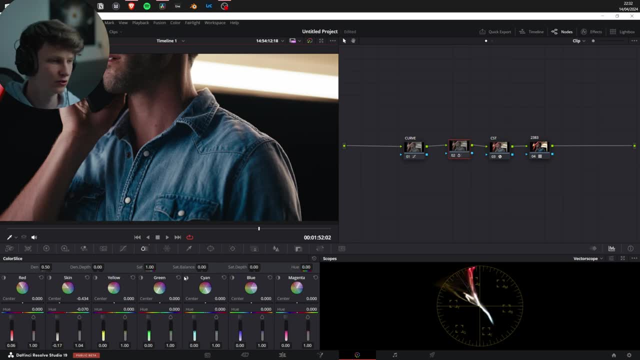 Though it's a light, so you should be a little bit careful. And then the main other thing I'm going to do is change this blue. It looks nice and normally you would do this in the color warper, but now you can do it here and it looks much nicer. So, as you can see, it's in the 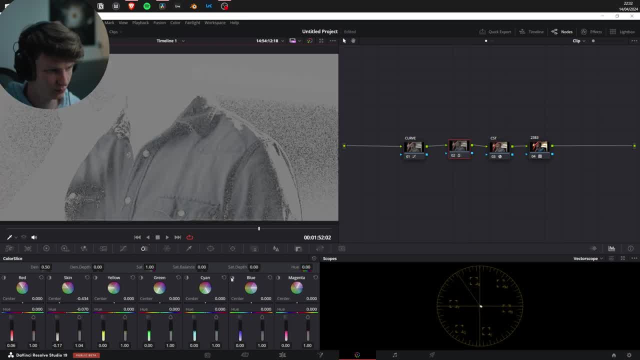 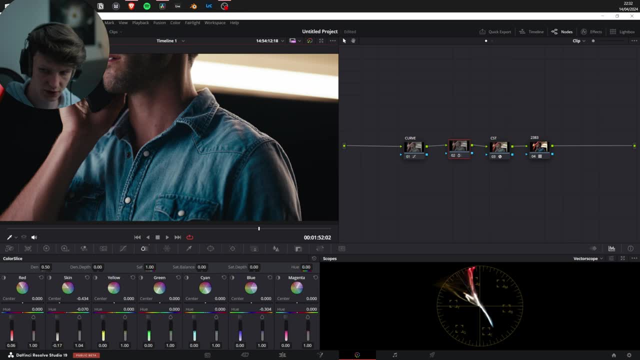 blue section mostly Cyan is obviously cyan, but we're going to go for the blue. It looks properly selected. so we're going to change our hue a little bit towards cyan, A little bit towards cyan, like 400 something, Yeah. Then we're going to remove a little bit of saturation- Quite a bit actually. 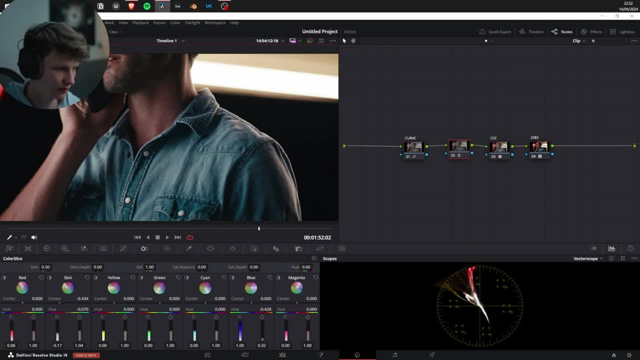 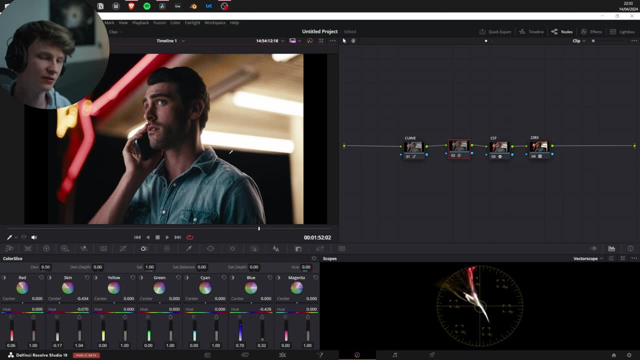 It's too much Right there, And then we're going to add up the density quite a bit because it looks really nice. Now we made our overall look go from this to this. As you can see, it looks way more filmic. It's absolutely insane that it's built in now, Because before you had to either download. 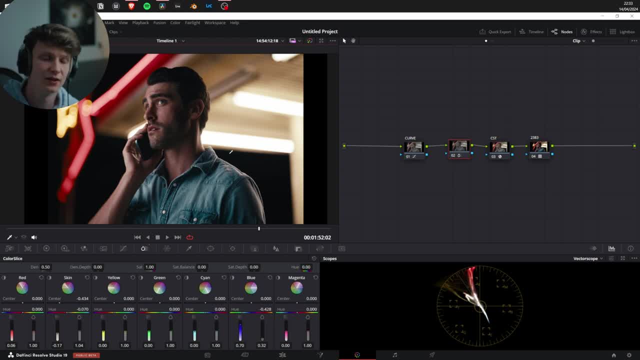 a free dctl, which I made a video about. All of you loved it. Now you can do it within Resolve itself, Or you would have to buy a dctl or plugin from a third party, And now it's built in It absolutely. 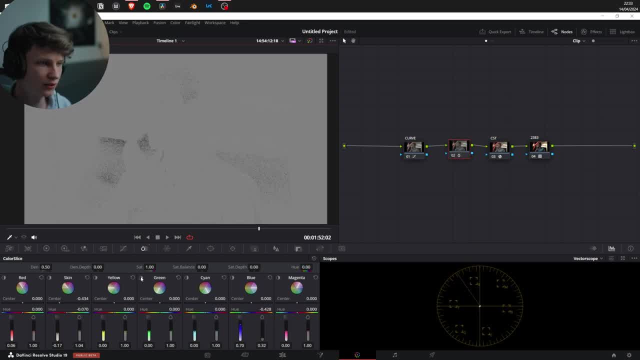 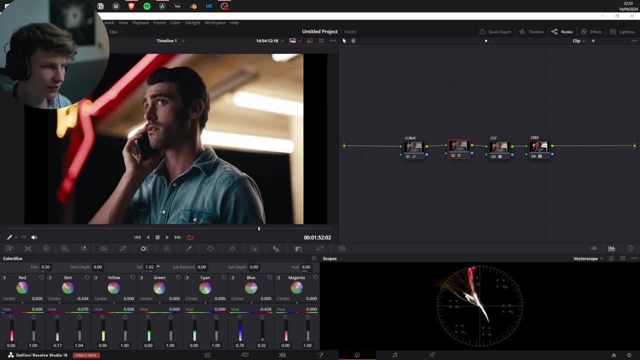 works amazingly, as you can see. I really love that you can choose where it affects the colors- These dctls, for example, Don't allow you to do that- And you have an overall depth slider. You can add some saturation and it looks amazing. We could also make a little bit of a change in the yellow if we wanted to. 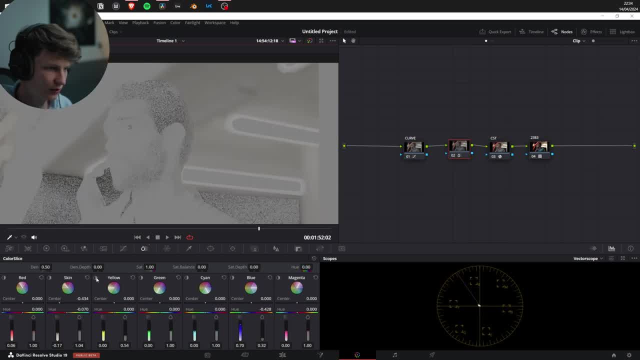 By lowering the saturation a little bit, Because when we look at the yellow, As you can see, when you press shift h it switches between the different sections you select. So we're going to go for yellow. I'm going to refine it to be: 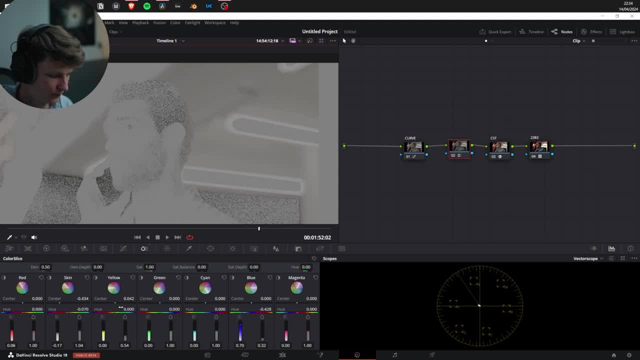 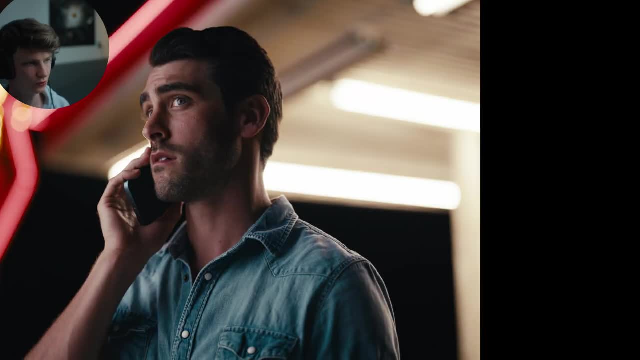 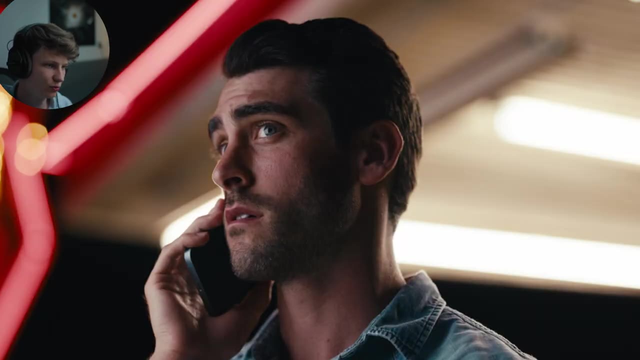 mostly the background. That should be fine. Shift h Desaturate it a little bit and it can be a bit lighter in my opinion. And now we also did that to the background. Sorry for it not being centered, But there we go. We went from this to this, Which in my opinion is a much more cinematic and pleasing.